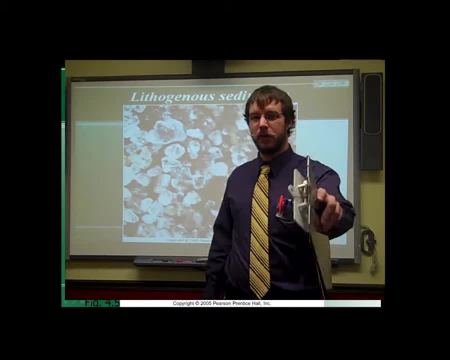 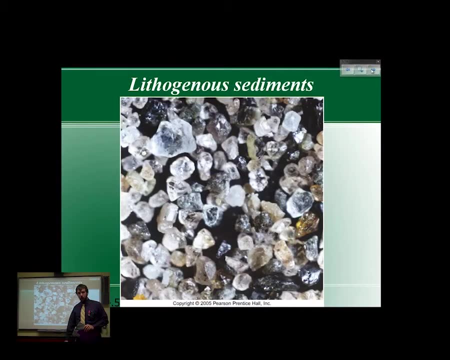 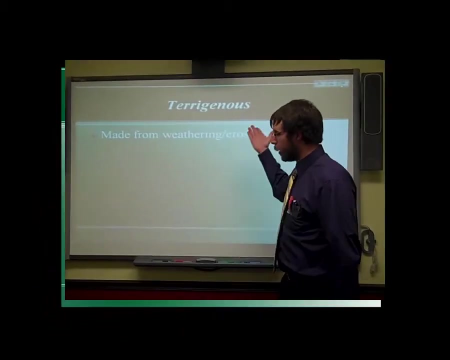 Lecture 1 out of 4 Sediments in Depth- Lithogenic Sediments. So here's a lovely picture of some lithogenic sediments. Remember these ones are from rocks, litho meaning rock. So these are broken down, eroded piece of rocks that are just crushed up and thrown into the ocean. all crushified, like Another name for them are teragenous, because they've been made from weathering and erosion. 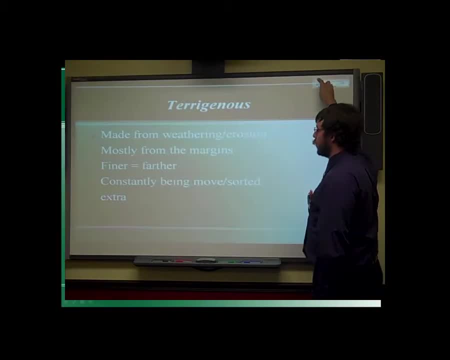 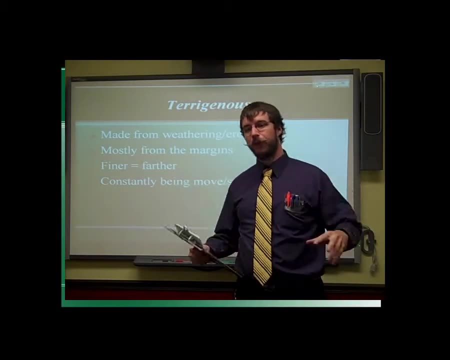 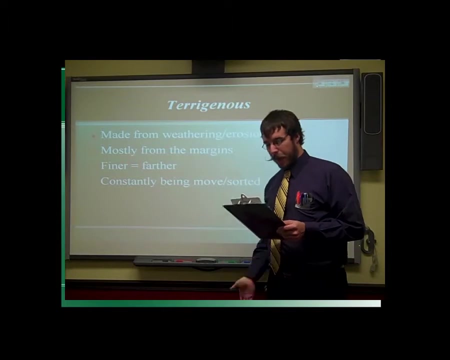 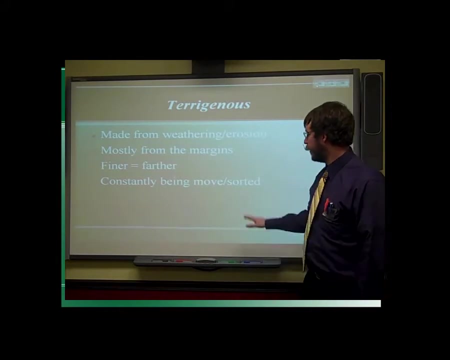 Remember, weathering is the crushing and erosion is the moving. Most of them are found in the margins. There's 22 billion tons of sediment every single year that gets put into the continental margins. In addition to that, 80% of Asia's goes right down the trench. So if you have an active conversion margin, you're not going to see a whole lot of that. 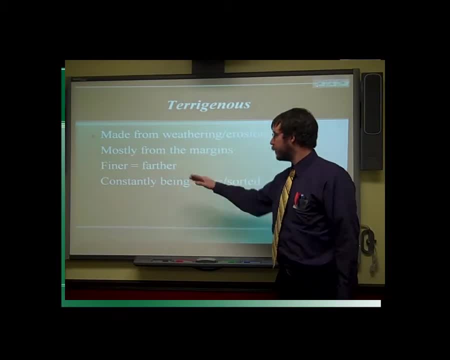 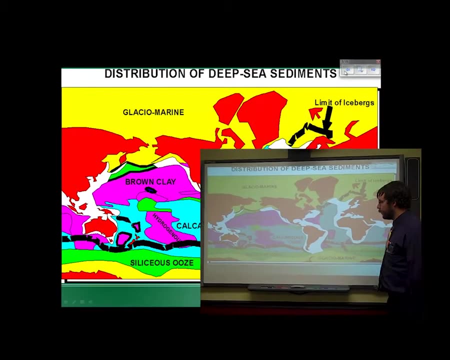 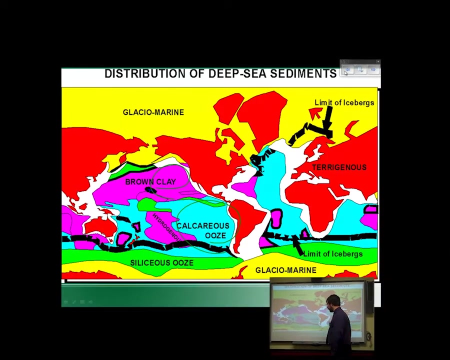 I remember it's constantly being moved and sorted and the finer the sediment is, the farther it gets. So here's a nice picture that just sort of demonstrates of where in the world you find different sediments. You'll notice that you see a lot of the word clay and a lot of the word ooze, which is one of my favorites. 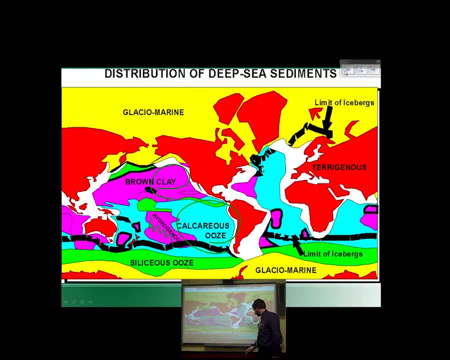 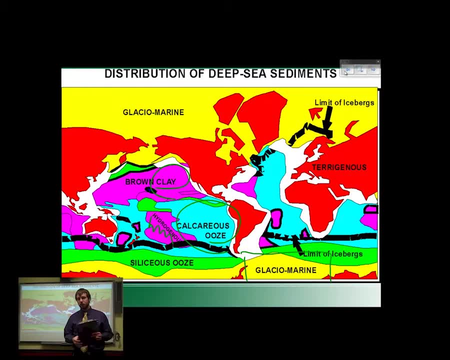 And then over here you have little pockets of hydrogenous sediment that we don't really care about for this lecture, Glacial and marine sediment. those are really fun because that's going to be a mixture of different glacial frozen pieces from the land mixed in with different marine pieces from the water. 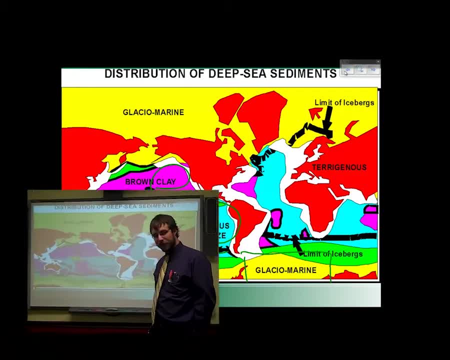 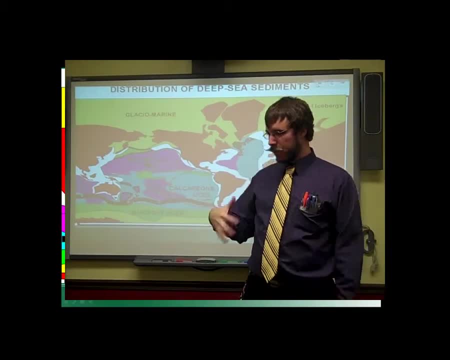 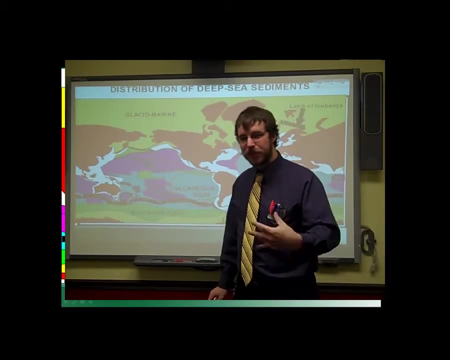 This is really kind of cool. It's worth noting now that ooze is a technical term. Think of like mud when it gets really like slushy and gooky. Think of like a slurry but it's made out of dirt, So it feels like ooze, but what it really is is microscopic pieces of sediment mixed in with water. 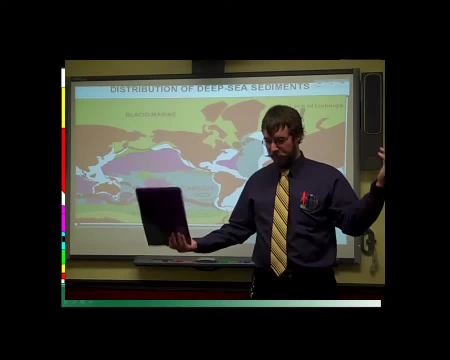 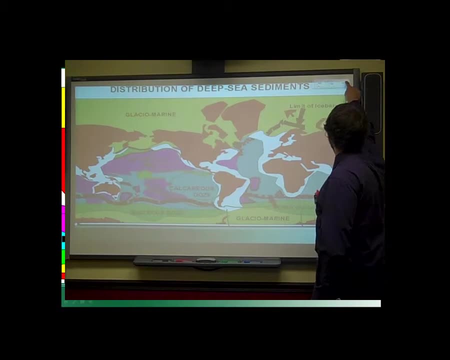 And so when you have that mixture it makes really like a fruit smoothie consistency. only you know, dirt and stuff Just gross. Clay, on the other hand, are even smaller. So here's a nice picture that just demonstrates that if you 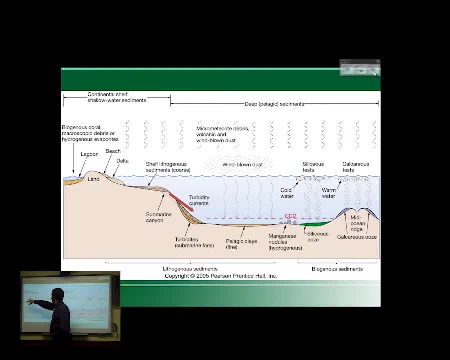 you've got sediment that's coming from the land and it's starting over here on the land. it will be carried at different amounts, mostly by the wind. You can see that some of it will also be carried by turbidity currents, taken right here off the shelf. 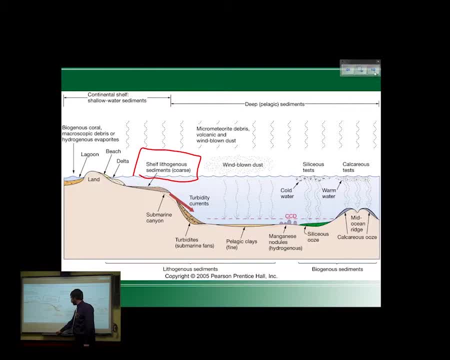 Those are shelf-lithogenous sediments because they come from the continental shelf And it'll make this turbidity current depositional fans down here. You also have different regions of pelagic clays, et cetera, et cetera. 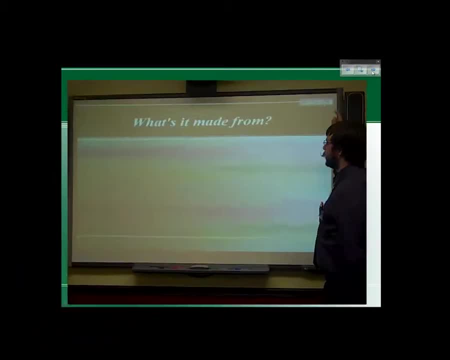 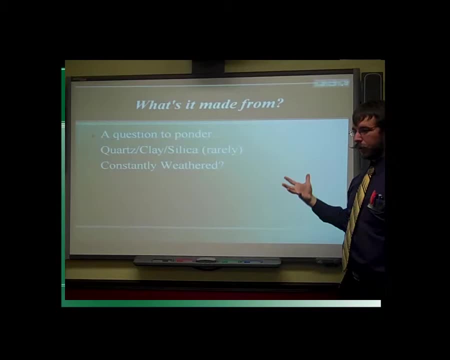 We're going to talk about these a little bit more in depth In a minute. For the most part you're going to have quartz-y stuff. You know it's going to be rarer to find because it's been weathered for so long. And so it starts as quartz, but it's rare to find because for the most part it's turning into other clay-like sediments. You'll find a lot of sand and gravel which is worth a fair amount of money, because with sand and gravel deposits you often find gold. 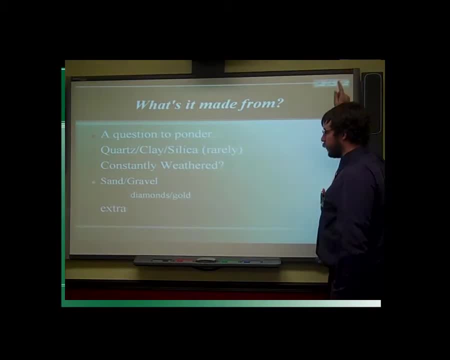 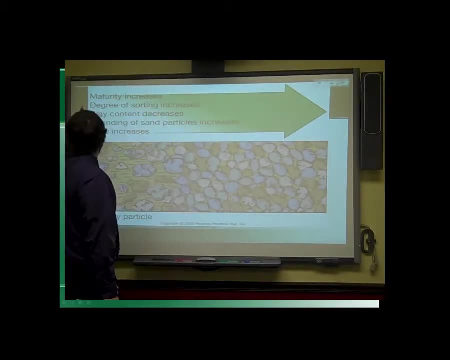 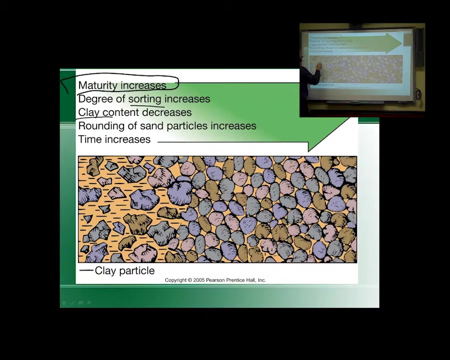 which is very important for, you know, gold, And you'll also find diamonds, which is a big deal. All right, we've talked about this one already, so we'll just hit it very, very quickly. Remember, as the maturity of the sediment increases, as the sediment gets older, it will become more assorted, more clay-like, more rounded. 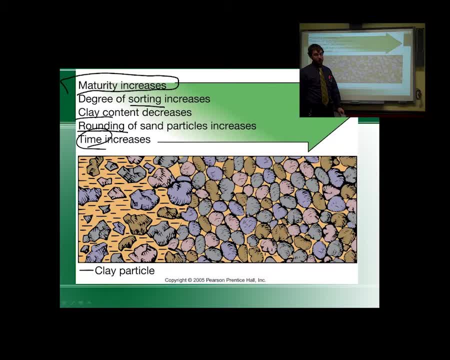 And that obviously happens as time increases, because that's the definition of getting older and more mature. So keep in mind that these sediments over here, on this side of the screen, these are the earlier ones that are assorted, These ones over here, these are angular. 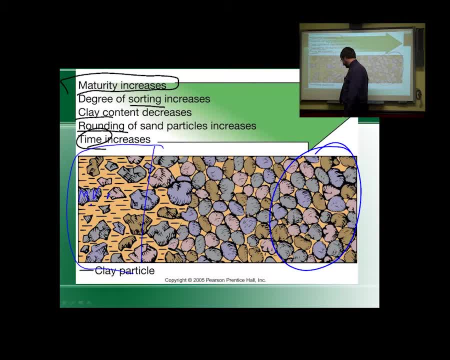 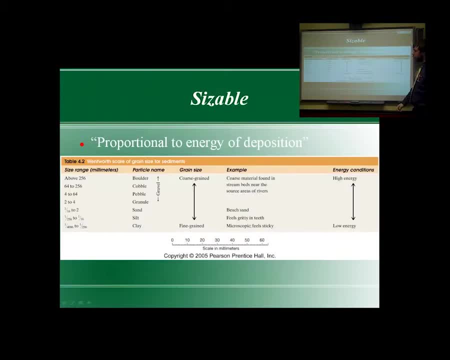 So you've got the big ones mixed in with little bits of microscopic things that you can't even see. Those would be an example of not well sorted. So here's the last table from Rubik's Table 4.2. It gives you the sizes. 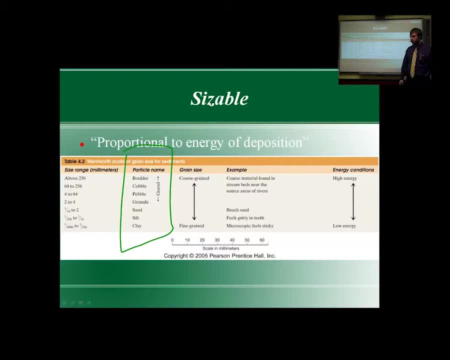 It gives you the acceptable names, for the sizes range big to small. You'll notice that they are in millimeters, which is really fun. So you'll notice that a boulder is anything bigger than 256 millimeters, which is 25 and a half centimeters. 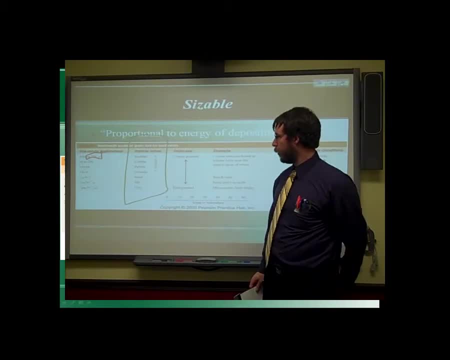 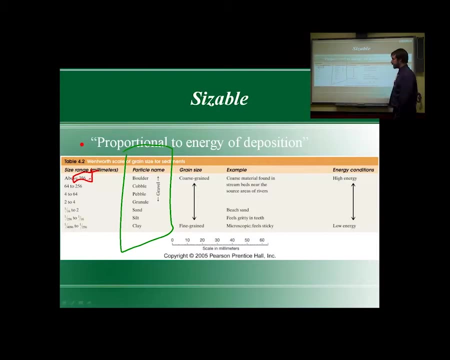 So you know, boulders are like that's a boulder. When we're talking about sediment size, It goes all the way down to the clay, which are 1,4096th of a millimeter. So these ones down here, the sand, are pretty small. 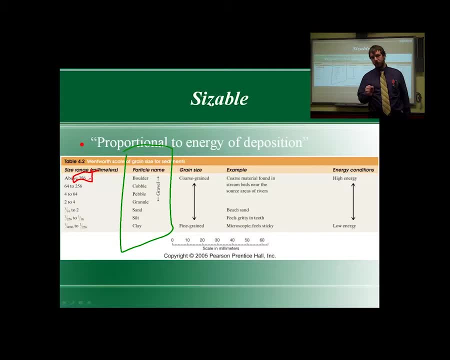 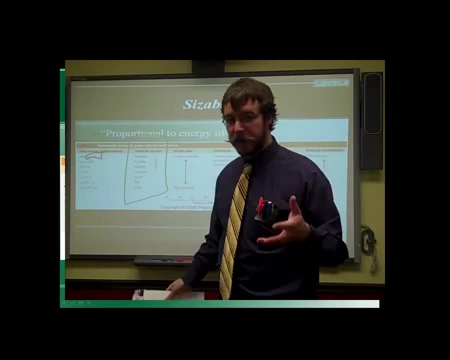 Silt and clay are going to be microscopic. You will not be able to see those grain sizes with your eye. When you look at clay, you see like there's a big lump of rock, but the geologist will actually see several different components. It's also worth noting that the larger the particle is, the more energy it's going to take to carry it. The smaller the particle is, the less energy it's going to take to carry it, Because the majority of marine sediments fall into this size range. They can be carried for a very long time because there's a lot of energy. So you can think about it the other way too. If you have a lot of energy, that means you can carry these smaller sediments much, much, much, much farther. 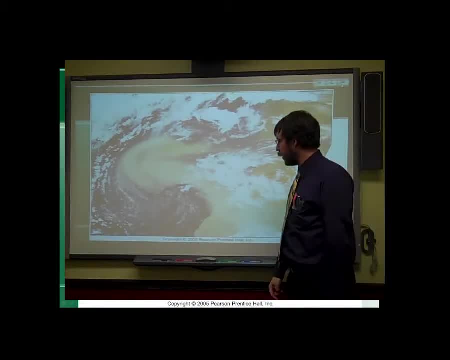 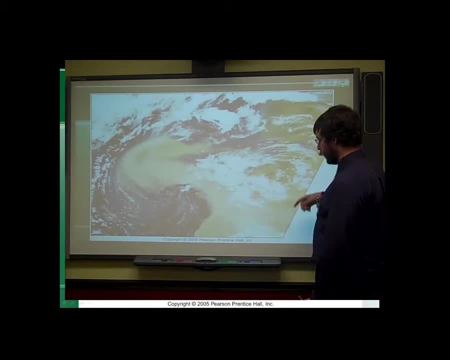 This is a pretty picturesque sediment you can carry. What is this? an actual? Well, this is satellite imagery. And then they drew some kind of sign here. This is coming off Africa. It's just dust There. it goes Out into the ocean. 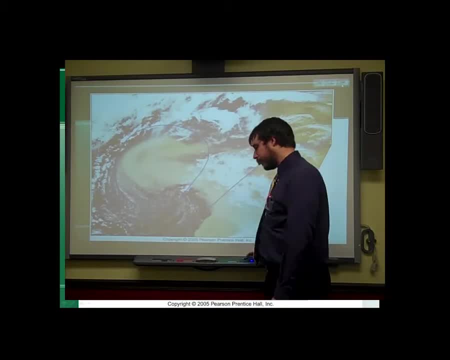 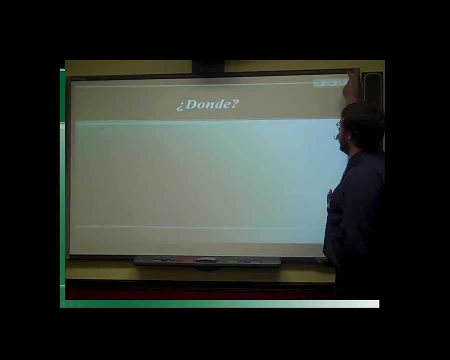 You notice, here is the mainland, Here is the dust cloud. It's still in there, So it's probably going to keep going. You'll not have the tendency to keep going once it's in the water, So you're going to find a bunch of sediments all over the place. 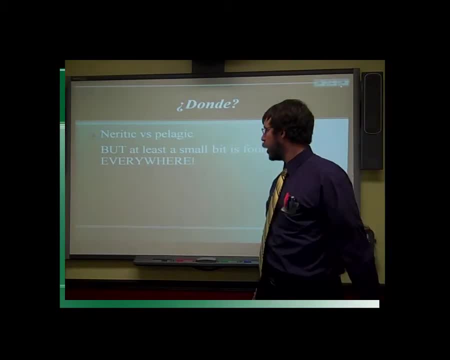 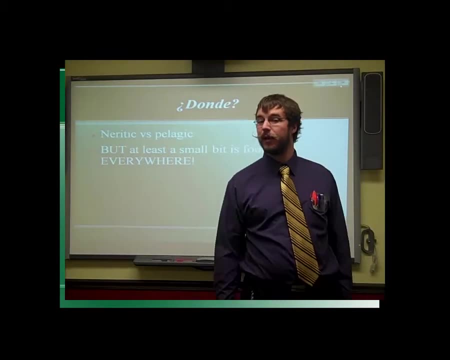 Now, before we go too much farther, I need to talk about the neuritic versus pelagic. Keep in mind again that you do find small bits everywhere. Anything that's neuritic, that's shallow water. that's technically a coastal region inside your continental margin. 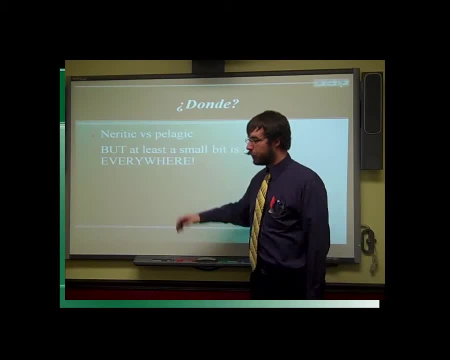 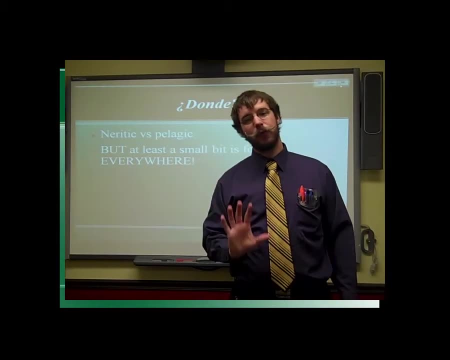 that would be the neuritic zone, Pelagic regions. that is, deep under the ocean's floor, that's in our deep ocean basin. So anything that we talk about being pelagic, those are found in the deep ocean basin. Anything that we talk about being neuritic. not neurotic, but neuritic. that is in the continental margin, So let's talk about neuritic sediments Again. the water is going to be shallow, The water is going to be warmer And you're going to be more likely to find lithogenous sediments. 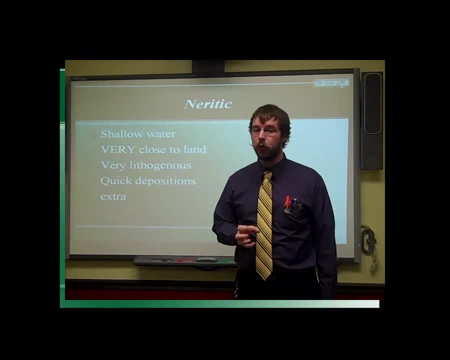 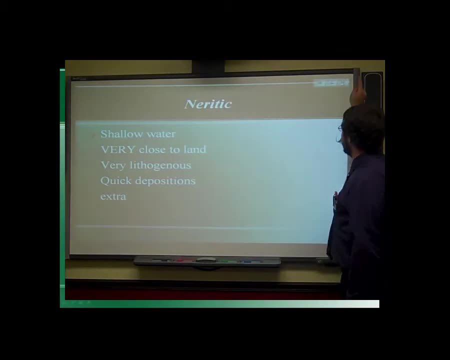 things that are deposited very quickly. Larger pieces are more likely to be found in your neuritic zone because, remember, it's not very far out. So these are the things that would need a lot more energy to carry them. You can find beach deposits anything up on the land. 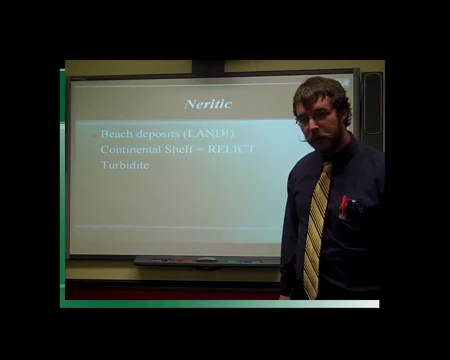 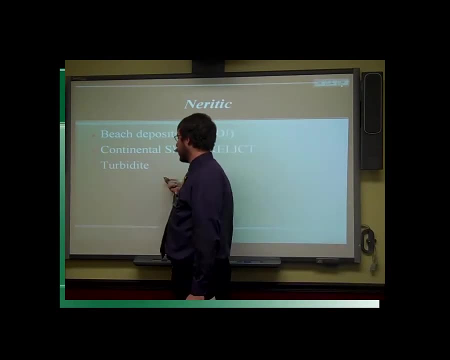 Things that are found on the continental shelf are actually called relict sediments, which is fun Think of like relics of the past, And then you also find our delicious and wonderful turbidite deposits. Those are also an example of a neuritic sediment. 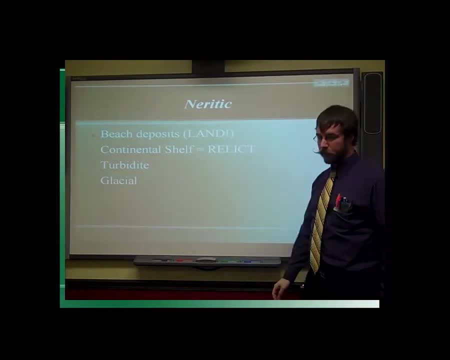 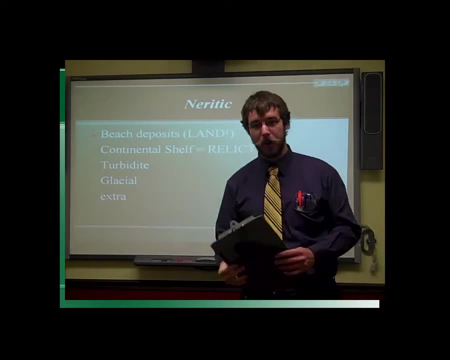 because they're deposited from the slope to the rise. Glacial sediments are very commonly neuritic because, you know, the glaciers are big and don't tend to go very, very far. I'm not talking about the ice itself, I'm talking about all the dirt and yoke and grime. 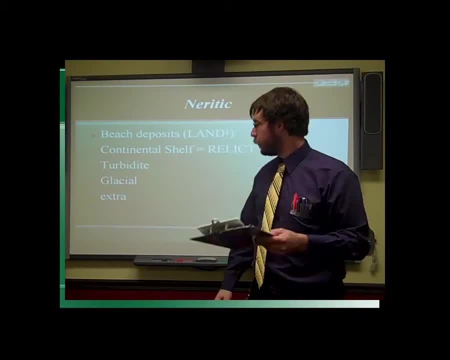 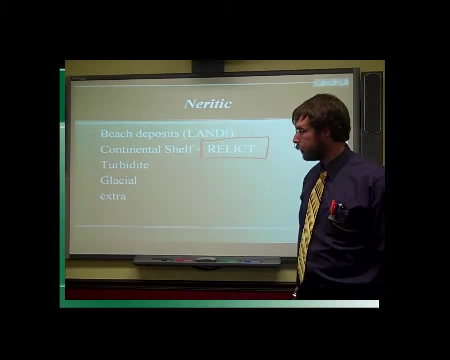 that the glacier is, you know, taken with it. It's worth noting that our relict deposits, those are in the ballpark of 3,000 to 7,000 years old. So those deposits from 3,000 to 7,000 years ago. 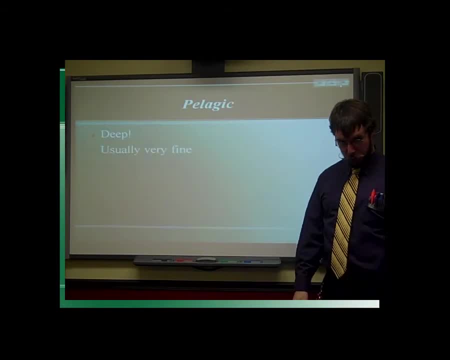 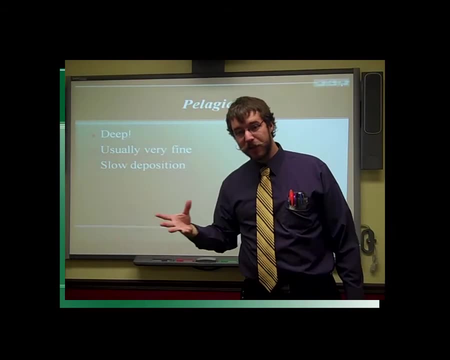 that's top pelagic. These ones are big. They usually tend to be very fine because, again, they've traveled a far distance, so you know they didn't take that much energy to keep pushing them As a result of their fine size. they take a long while to settle through the ocean. Remember, salt water is relatively dense, so it's going to take a little while for these things to get through. even though that they are relatively dense compared to normal water, It'll take them longer to settle to the bottom. 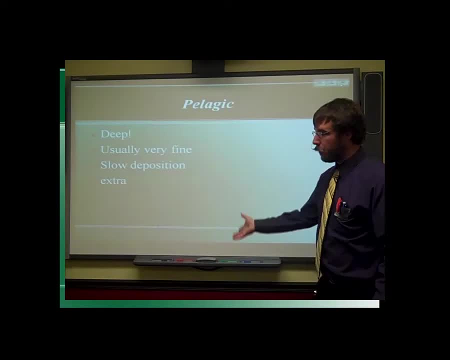 Plus, you have currents and, like things, swimming Ships and marine creatures like mermaids swimming around in there, So they take a little while to get down to the bottom. Some examples of pelagic sediments are your abyssal clay. They tend to be very rusty in color. 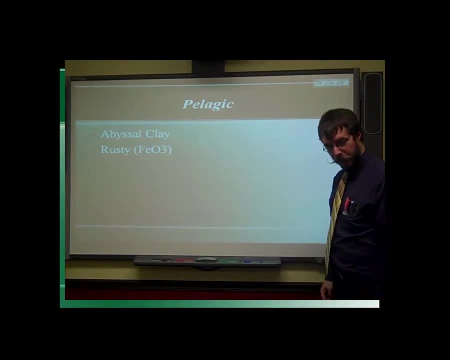 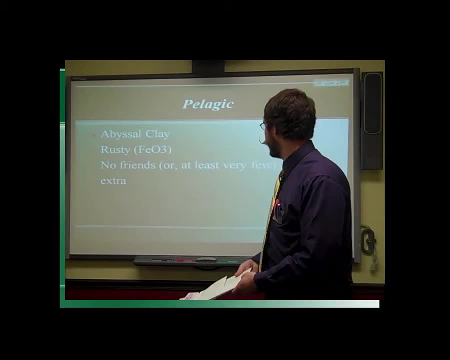 because they've got a lot of iron oxide, which is rust. by the way, The only type that we ever have that we call it are abyssal clays. That's it. That's all you really find there. So here are some of the key players that are going to be carrying. 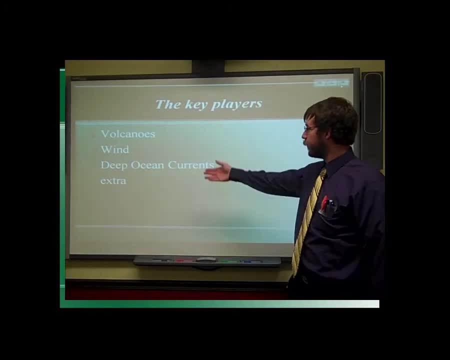 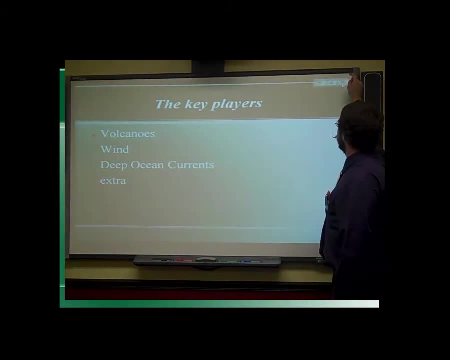 These are the erosional elements carrying the sediment force. You've got stuff coming out of volcanoes, stuff that's blown by the wind and stuff that's carried by deep ocean currents. Volcanoes are a very interesting one because it gives us a good idea of different natural disasters, etc. 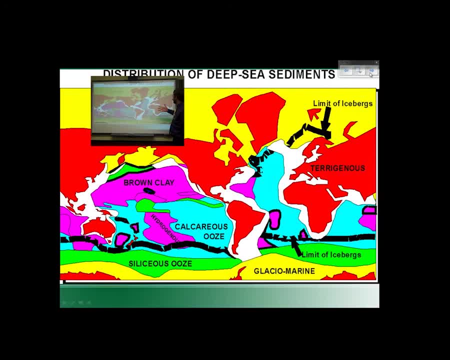 So you can see here again. now that we've talked about those things, I want you to just ponder on the map and then you can see. So we've got you know, here's America, Here's Eurasia, over here. 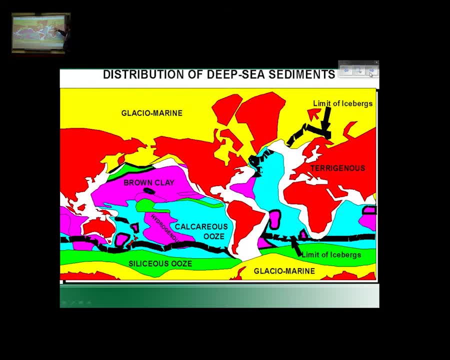 So Europe's sticking off somewhere over here, But you can see there's Africa, But you can actually see there's big zones where you find different lithogenic sediments just throughout the ocean, which is really kind of cool. Keep in mind all these sediments, the lithogenic ones. 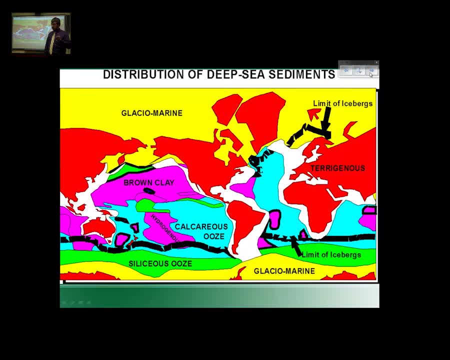 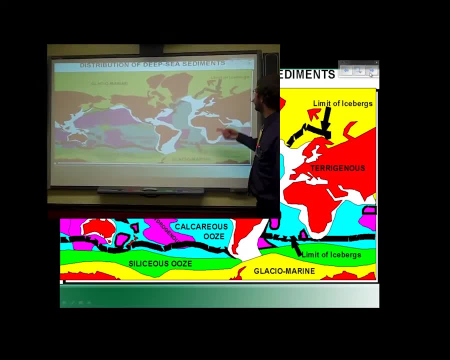 all started on the land, usually mainland big continents, and they go out into the ocean for a pretty good amount of space. If you have any questions, go ahead and put them in the forum. But that's it for lithogenic sediment.